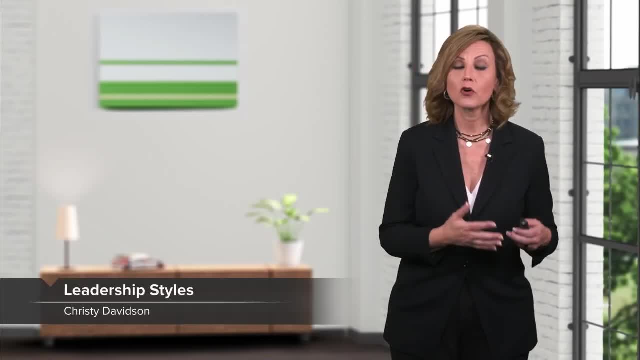 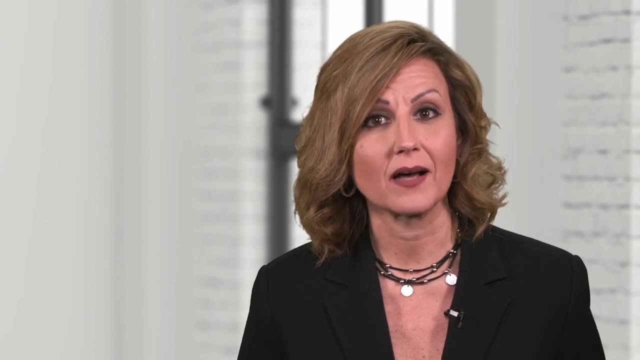 Welcome back everyone. Regardless of whether you are a formal leader or an informal leader, you are going to have your own way of expressing yourself. Today, we're going to be talking about leadership styles. Now, it's important to know that different leadership styles are. 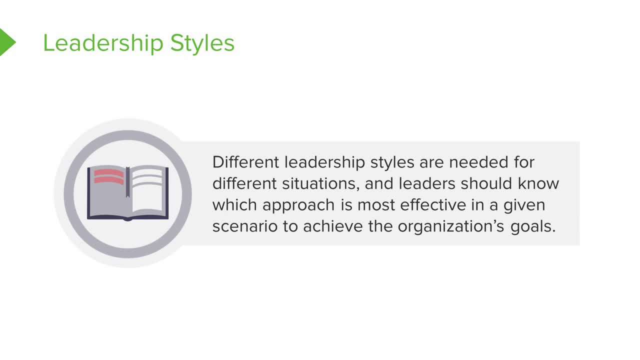 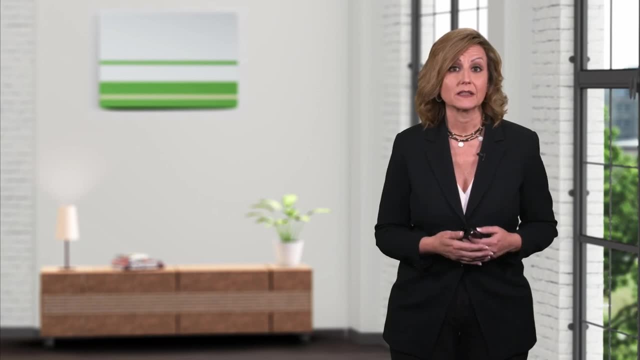 needed for different situations, and leaders should know which approach is most effective in a given scenario to achieve the organization's goals. Now, there are three classic leadership styles. The first, authoritarian. This is where a leader makes all of the decisions without really 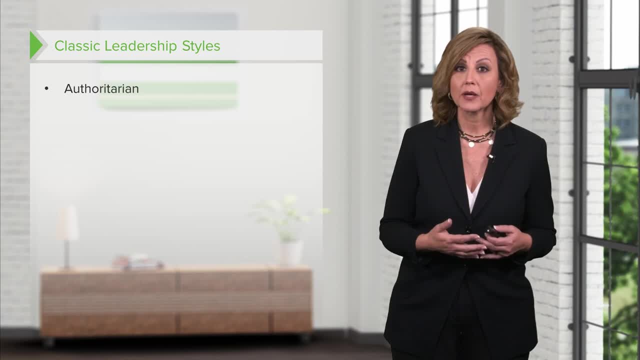 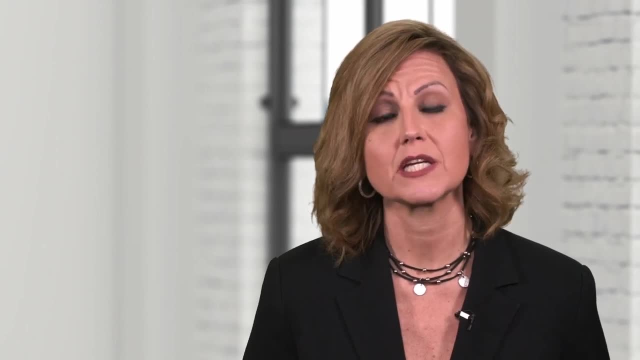 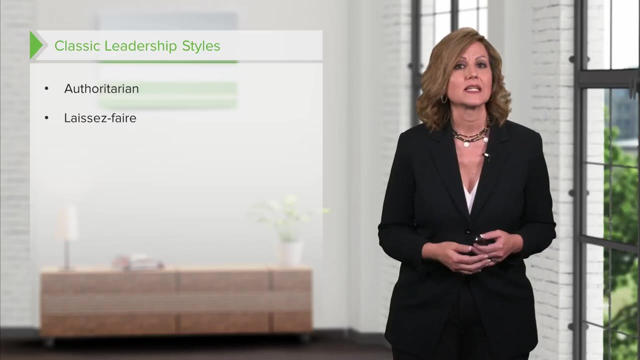 considering input from the staff. Negative reinforcement and punishment are often used to enforce the rules. Now, this doesn't always have to be a bad thing. Sometimes this particular leadership style may be effective in an emergency where quick decisions need to be made. The second one is laissez-faire. This is where the leader provides little or no direction. 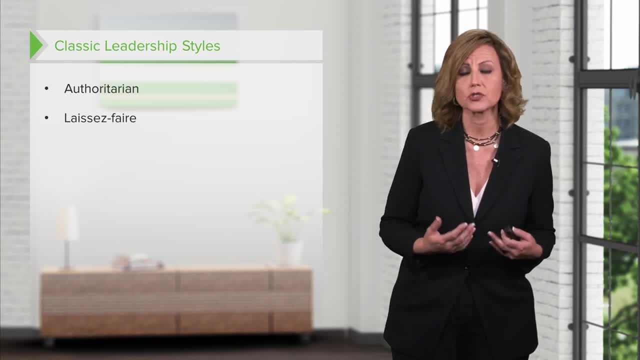 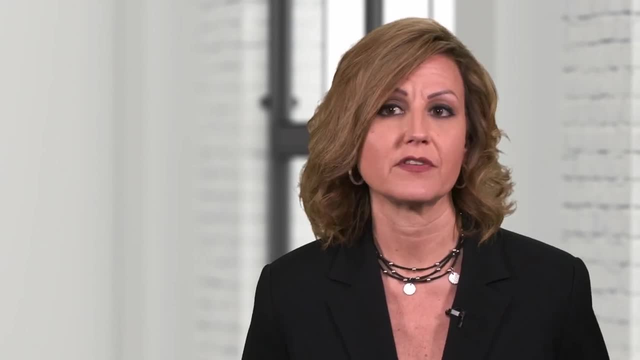 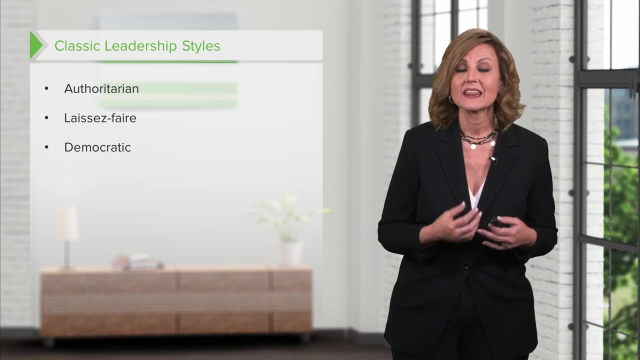 or supervision and prefers to take what we think is the most effective approach. This is what we call a hands-off approach: Decisions are not really made, changes rarely occur and quality improvement is typically reactive, meaning after the fact, not proactive or forward-facing. And the third one is democratic. This particular leadership style really encourages. 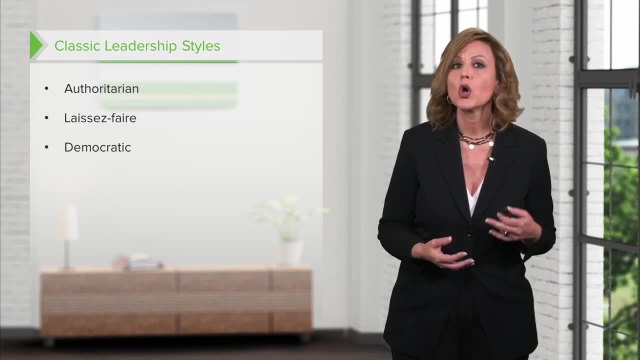 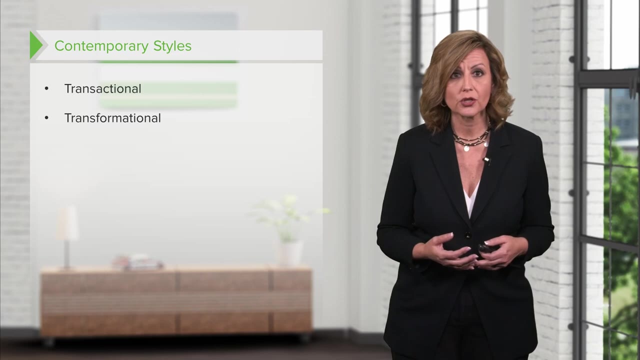 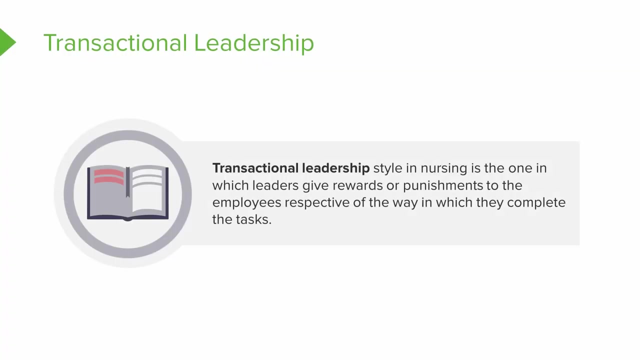 open communication and staff participation in decisions. Workers are given responsibility, accountability and feedback regarding their performance. Now there are several contemporary styles that we want to discuss today. These are transactional, transformational, servant, authentic and visionary. The first one is transactional: Transactional leadership in nursing is the one. 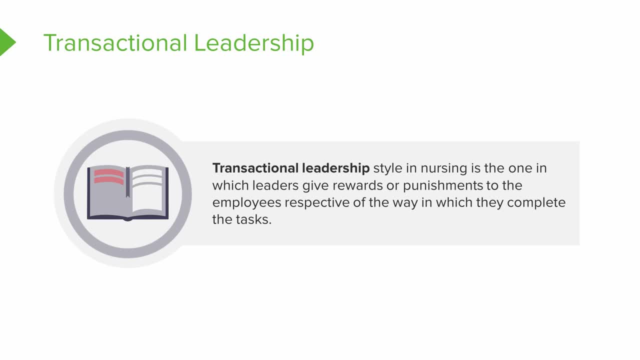 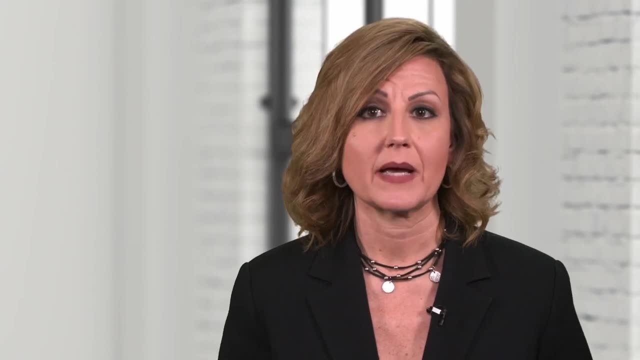 where leaders give rewards or punishments to the employees respective of the way they complete the tasks. Now, different from transactional, leadership is transformational. This style in nursing is based on the encouragement and the feedback regarding their performance. This style is based on the encouragement of the employees to give their best at work. 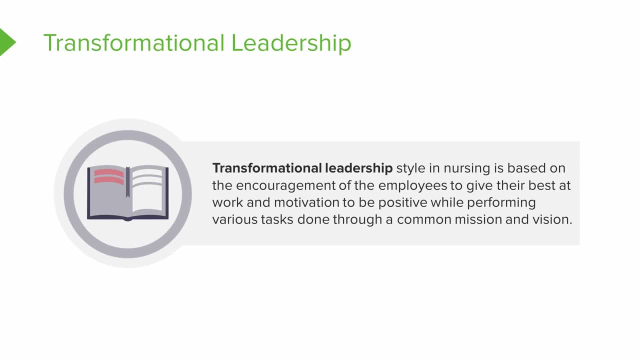 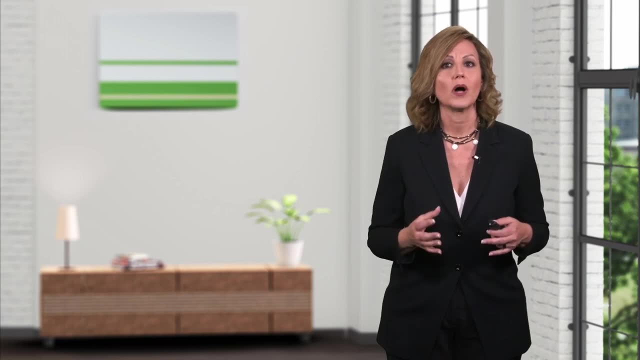 and motivation to be positive while performing various tasks done through a common mission and vision. Another one is servant Servant leadership style in nursing is the one which the main goal of the leader is to serve. A servant leader shares the power, puts the 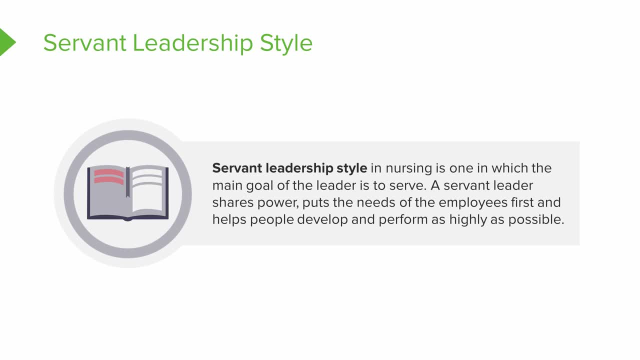 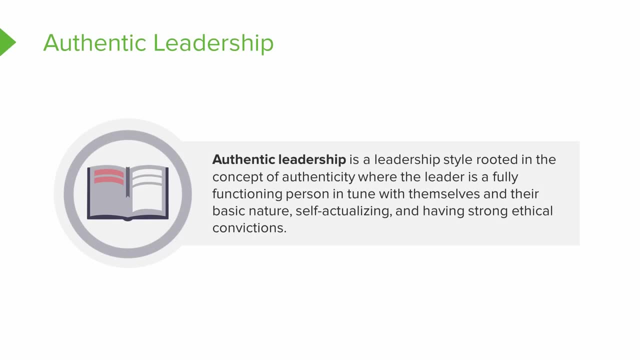 needs of the employees first and really helps people develop and perform as highly as possible. Next, authentic leadership. This is a leadership style rooted in the concept of authenticity, where the leader is the one who is the leader. This is a leadership style rooted in the concept. 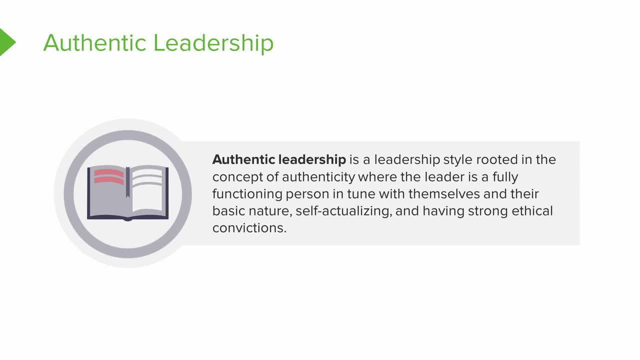 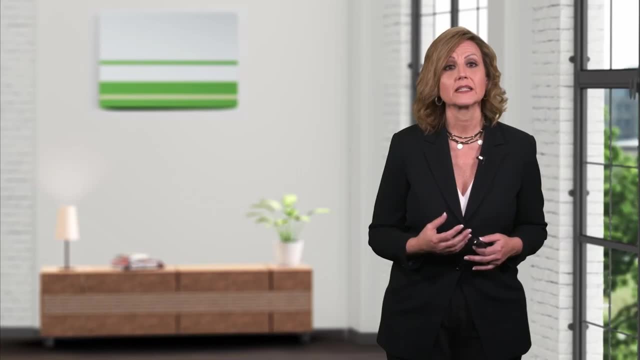 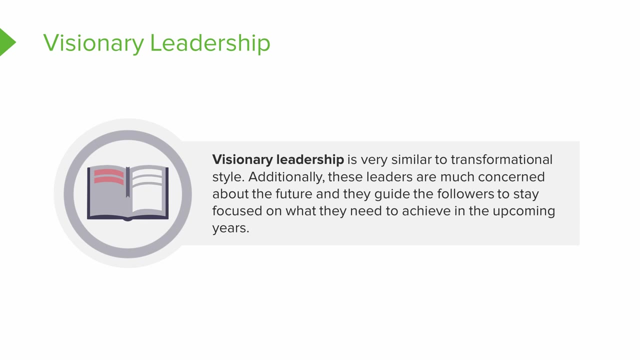 of authenticity, where the leader is a fully functioning person, in tune with themselves and their basic nature, self-actualizing, and they have strong ethical convictions. And, finally, visionary leadership. Now, this is very similar to transformational. Additionally, these leaders are much concerned about the future and they guide the followers. 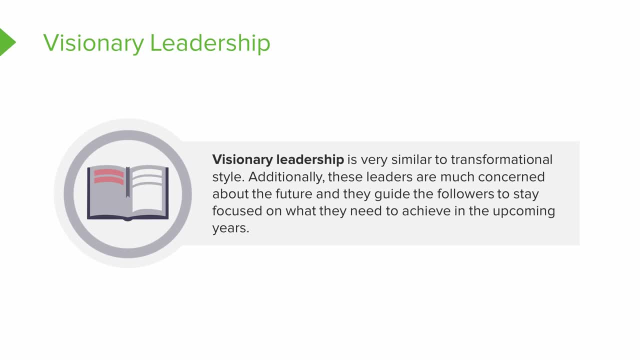 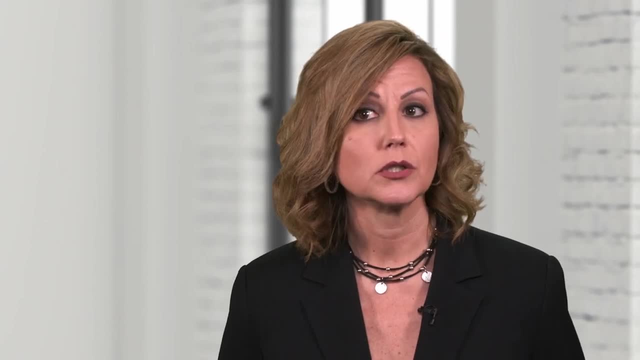 to stay focused on what they need to achieve in the upcoming years. So here's a great example for us to go through. Pat is a nurse manager for the operating room of a small local hospital. She's a nurse manager for the operating room of a small local hospital. 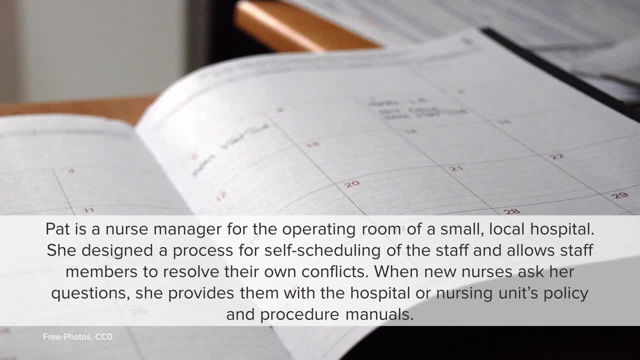 She designed a process for self-scheduling of the staff and allows staff members to resolve their own conflicts. When new nurses ask her questions, she provides them with the hospital or the nursing unit's policy and procedure manuals. Which type of classic leadership style is Pat? 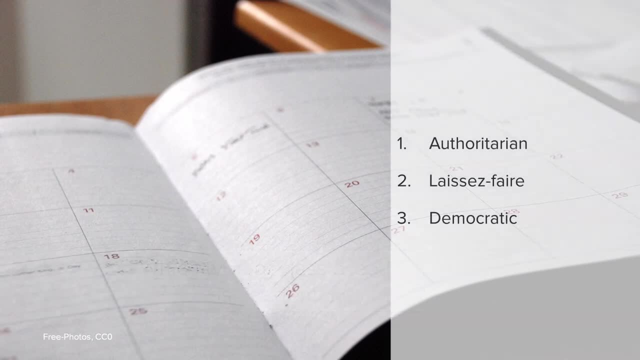 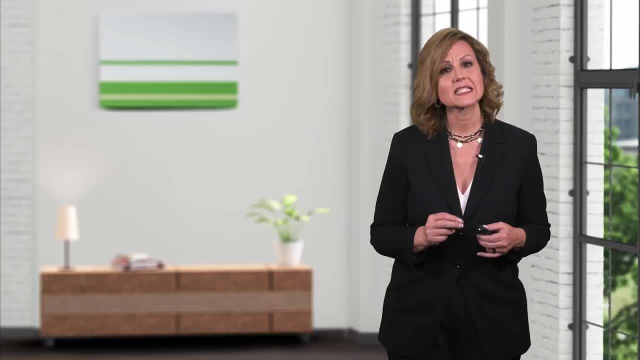 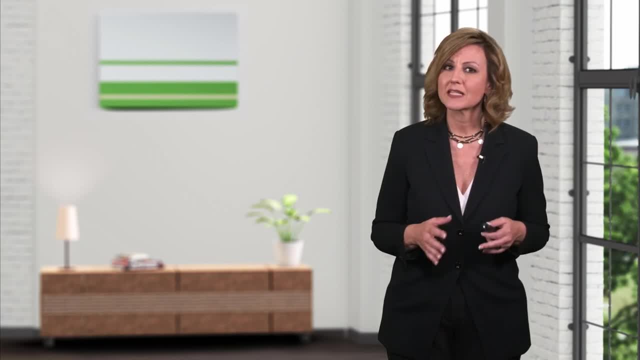 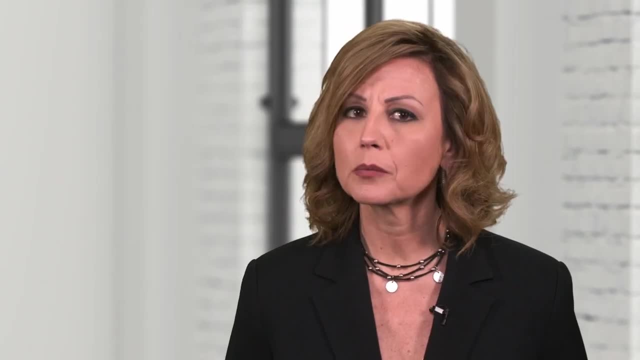 own schedule. She does not do that for them. She also doesn't intervene when they have conflict, so she doesn't act as a mediator or a liaison there. And third, when a new employee asks for help, she simply gives a policy and procedure for them to read, rather than spending time with them. 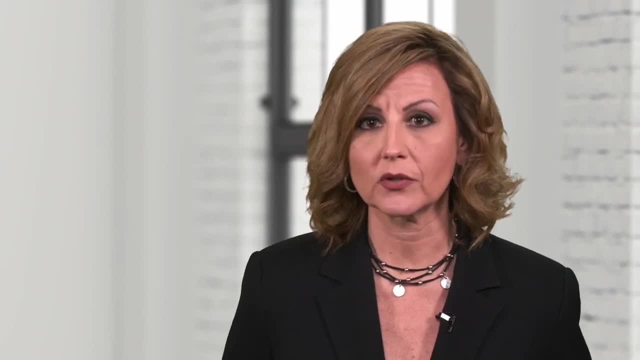 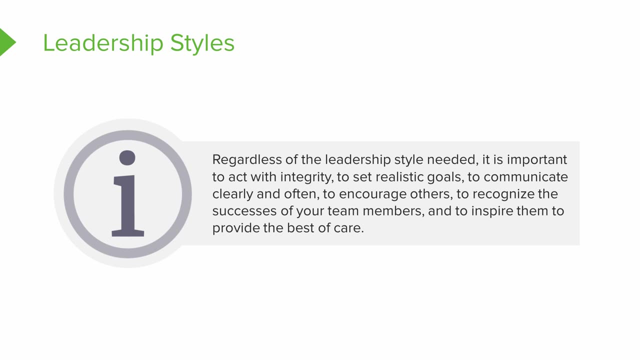 and really teaching and coaching them on what they need to be successful in the unit. So remember, regardless of the leadership style needed, it's important to act with integrity, to set realistic goals, to communicate clearly and often to encourage others to recognize the successes. 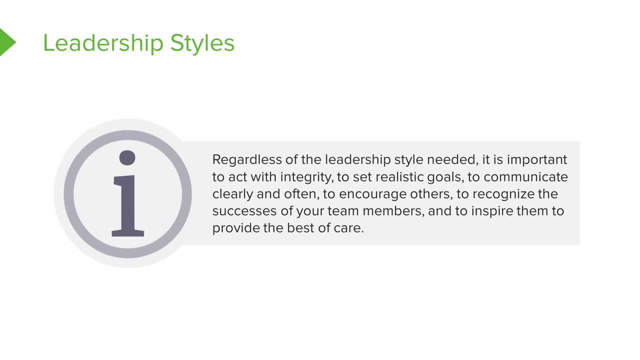 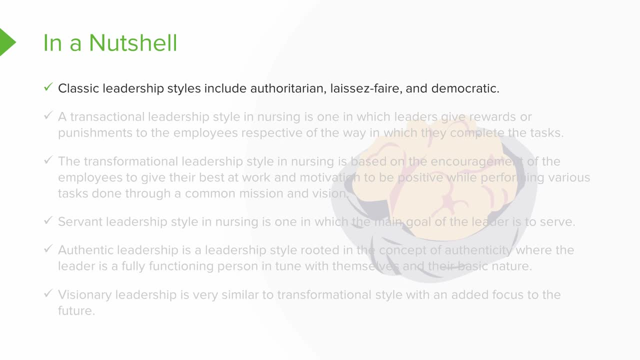 of your team members and to inspire them to provide the best care. So what did we learn today? First, we learned classic leadership styles include authoritarian, laissez-faire and democratic. The transactional leadership style in nursing is the one which leaders give rewards or